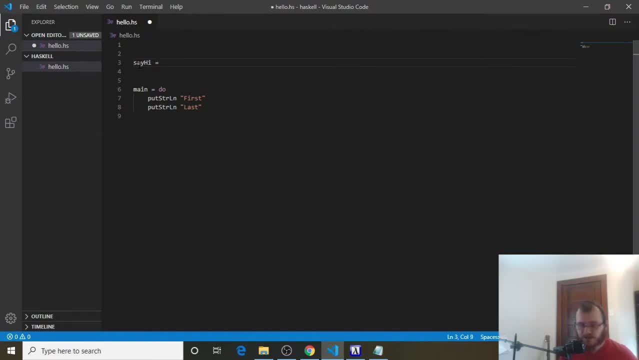 the function, And we're going to give it a name, And we're going to give it a name, And we're going to give it a name, And I'm going to say equals, And the right-hand side of the function is what? 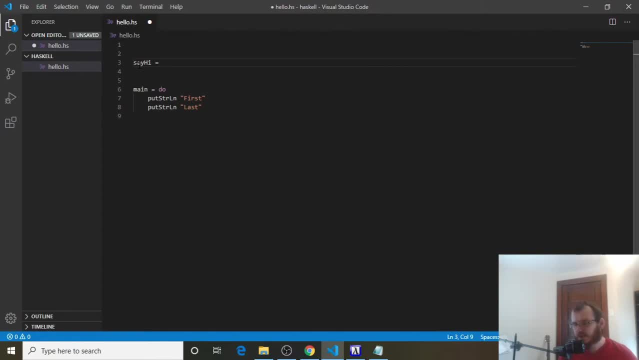 happens when we call say hi, the name say hi. So on the right-hand side we want to put string ln And we're going to say hello user. And our function kind of describes what it does, right. So say hi is the name of it And it describes what the right-hand side does In this case. 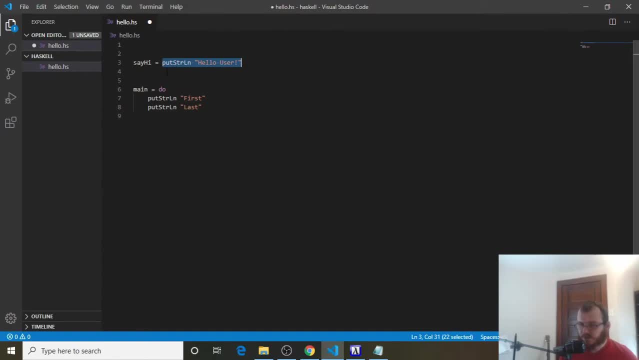 it puts to the console: hello user. So that's our function. Remember, we only need do if we were to print multiple things, So we could say do and then print multiple things, But we're not going to do that yet. So if we only are putting one thing to the 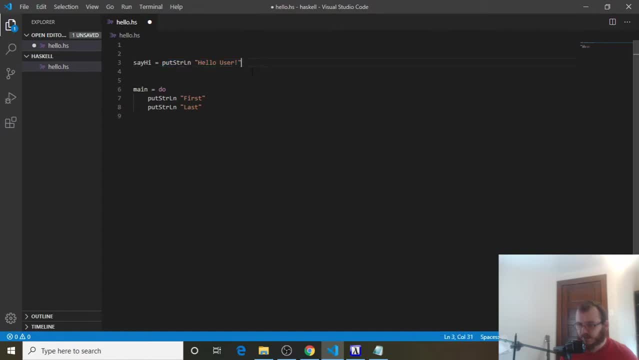 console, we can just say it equals this And let's save it. And this is now: we have our function, but it's not going to run because we never call our function. So let's just take a look at that and make sure. What we should get is this main function evaluated, And it should just put first. 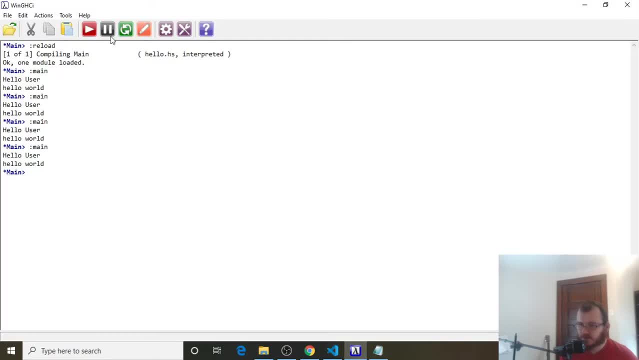 and last. This is here but it never gets evaluated. So let's go over clear it, refresh and evaluate main And you're going to see it prints first and last. And the reason it does that and it doesn't call this is because we never said in this main: 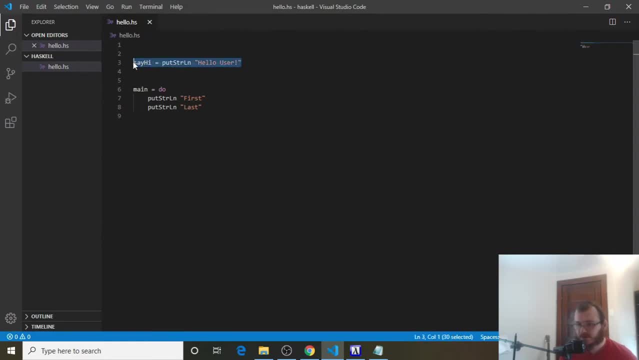 function. hey, we want to call this function. We just declared it. So we said this is a function, but we never said when we're going to call it. So to do that, we can come in between first and last And we call our function by just typing say hi And that will call this: say hi function. 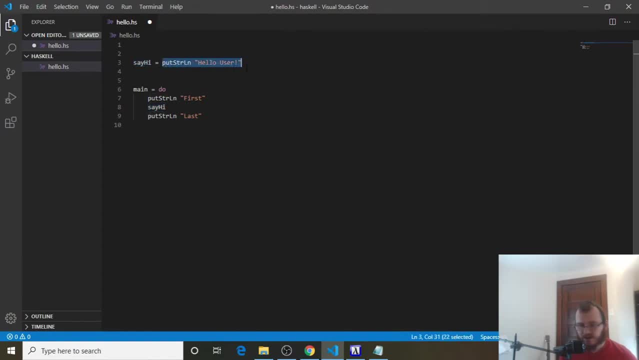 And it's going to do whatever is on the right-hand side of that function. And you'll notice I put it between first and last. So remember the main function, the do function. it prints everything in order from top to bottom, So it'll start with this, Then it'll call this: say hi. function. 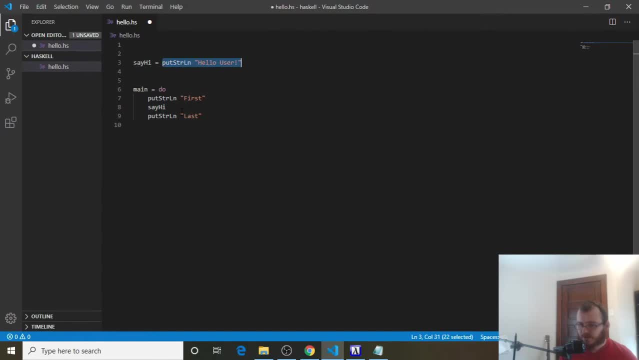 which will put hello user to the console, And then it's going to jump back down here to put string ln And it's going to put last. So it'll be first hello user, because we're calling this, and then last. So let's save it with control s. 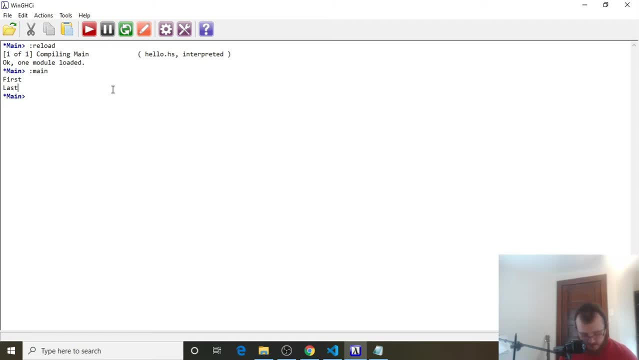 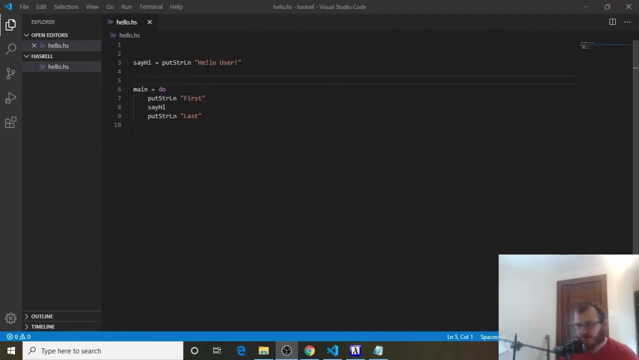 head over to win GHCI and we're going to clear it, refresh and evaluate main. And so we have first, hello user and last. So there we've written our first function in Haskell. Now we're going to use this say hi function to do multiple things. So if we want to print out, 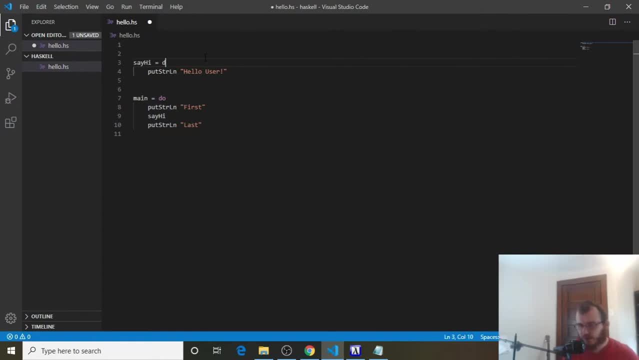 multiple things with a function. we're going to put do function and then we're going to put do on the right-hand side and then we're going to put the things we want to do underneath the function. So in this case we want to put hello user. 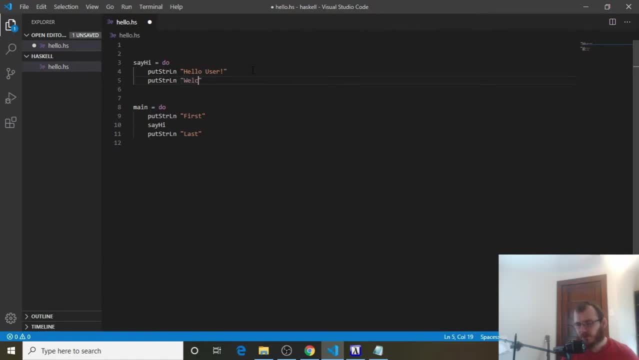 Then we want to put let's go with welcome. And so now we're doing two things: in say hi, We're putting hello user and then welcome. So this is the order right. So it evaluates main when we push the red button and then it puts: first It runs, say hi, function and it runs. 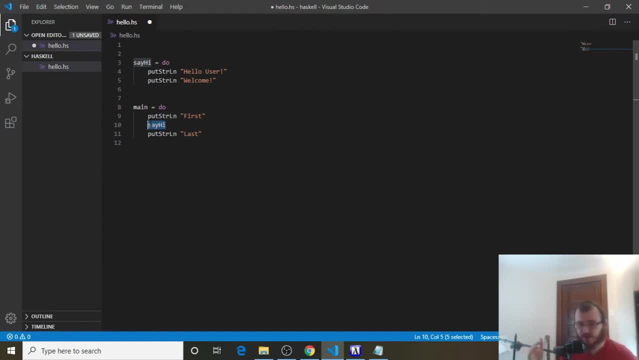 everything inside of say hi function. It doesn't just go to the next one after does one step. it runs everything. so it comes up to say hi and evaluates everything on the right hand side slash underneath the function. so in this case it's going to do first, then it's going to run. 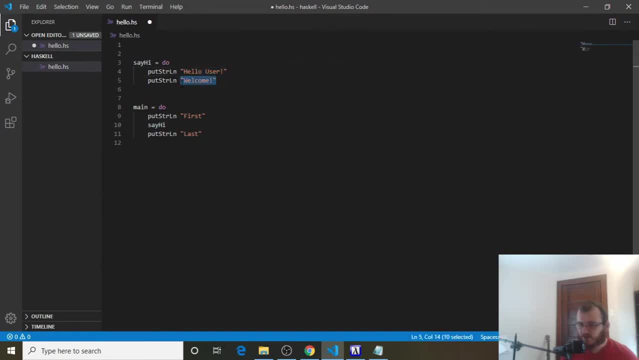 say hi and it's going to put hello user. then it's going to put welcome. then it's going to jump back down to main, because it's out of instructions, and say hi. once it gets to the bottom of this and there's nothing left, it's going to come back to main and it's going to put last. let's test that. 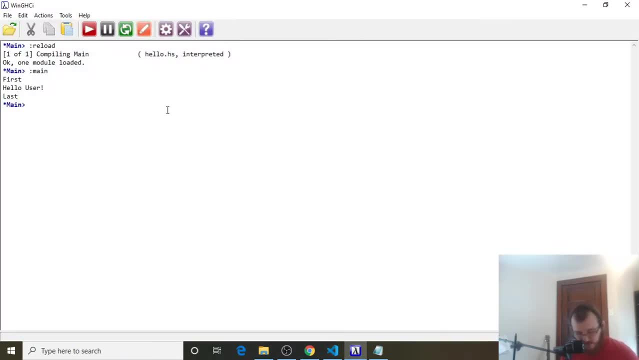 ctrl s to save, head over to win ghci. clear it, reload it, refresh and evaluate main. you're going to see it does first. then hello user. we're in the say hi function. now, then welcome. and then it prints last: okay, so that's multiple things in the say hi function. now let's take a second to talk. 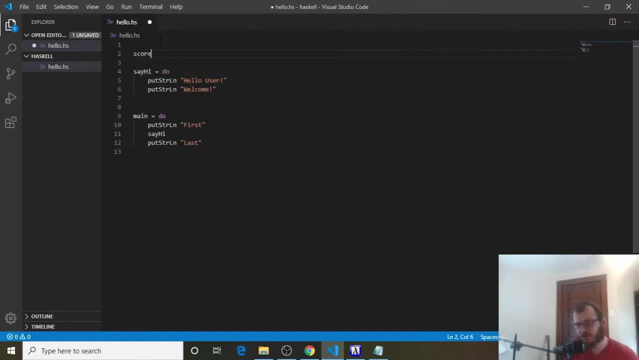 about types with our functions. so when we made variables right and we said score equals 30, and we know 30 is an int, right, an integer, so we can say score, colon, colon, int, and we're saying that, hey, score is going to be an int. and then we declare the int and set it equal to score. now we're going to do something really. 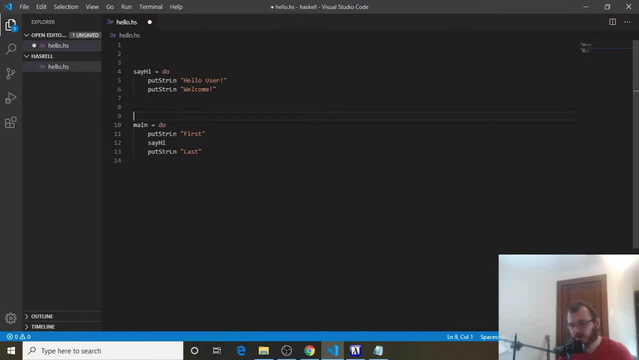 similar with functions. in this case, our main function is always going to return a specific type. we haven't talked about this type yet, but we're going to right now. so we're going to say main above our main function, right, just like we did our variable up here. so i'll type this back. 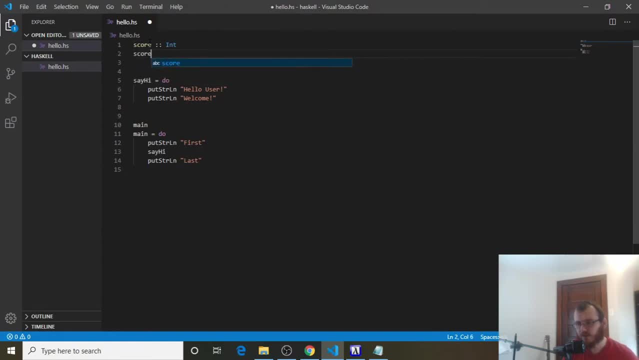 in just for clarity: score int. now we set score to 30.. so we have main equals do and above main we want to set the type of this function, and this is called a return value. we're going to talk more about return values in the next video, but for now we're going to set it equal to a function called. 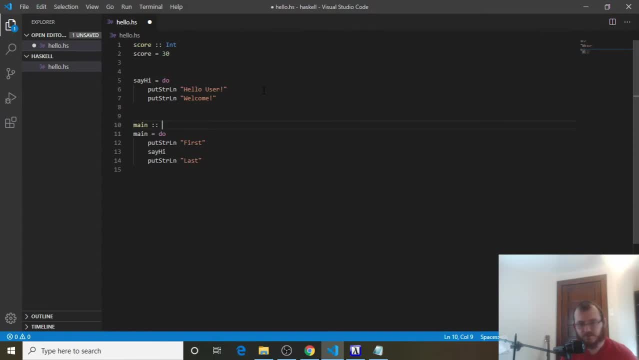 io and that just means we're printing or putting something to the console for now. so if we're printing or putting something to the console inside of our main function, we're going to set it equal to a function which is going to be almost always. we're going to say io and then we're going to add: 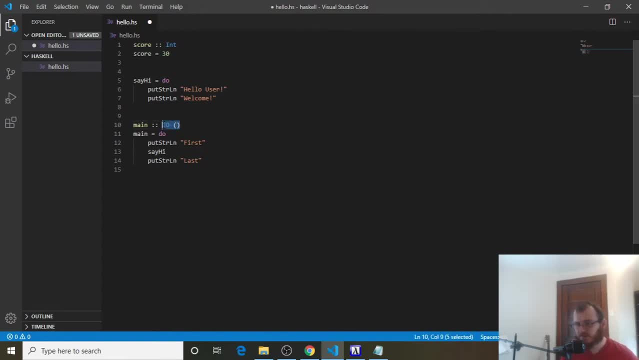 parentheses on the end. so this is a bit confusing, but for now this means that we're going to end our main function with printing or putting something to the console, and you'll notice up here now we need to type out: say hi, because we haven't done this yet. right, it's also a function. 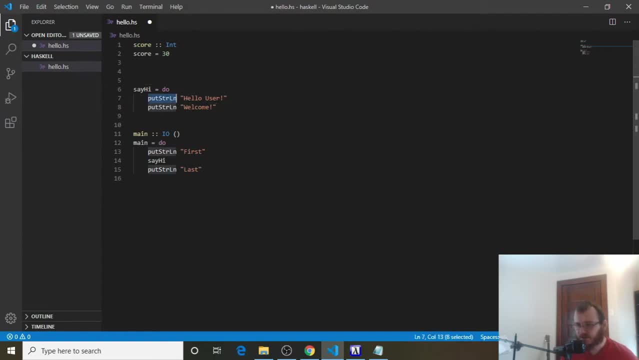 and what are we doing in this one right, we're still putting something to the console, so it's going to have the same kind of function definition for it. so say hi, colon, colon. and this, the last thing in the say hi is we're putting something to the console, right? 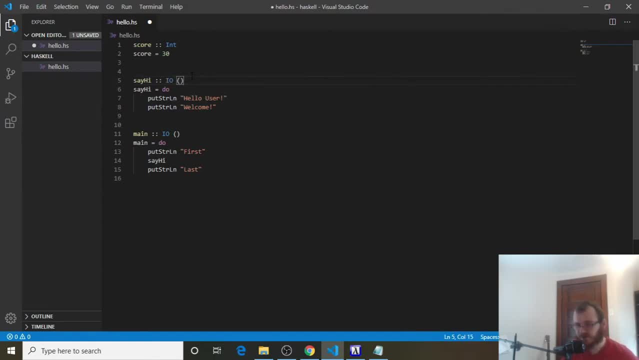 so it's still going to be this io type with these parentheses. even if it were just one thing in say hi and we're still putting it to the console like this, the type would still be io, because we're still putting something as the only thing we're doing inside of it to the console. i'm going to put those. 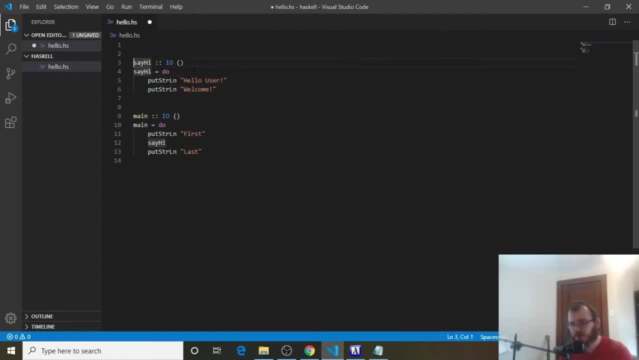 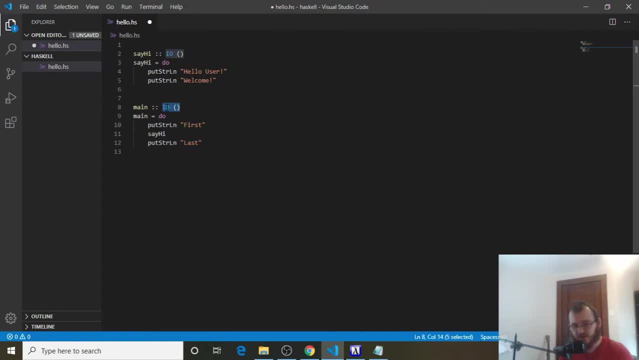 console and we said that is how we declare, that is io, and then parentheses, and then the same thing for zehi. because we're doing the exact same thing. the last thing in say hi is putting something to the console and we're saying it's going to do that by writing io and then parentheses, ctrl s to save. 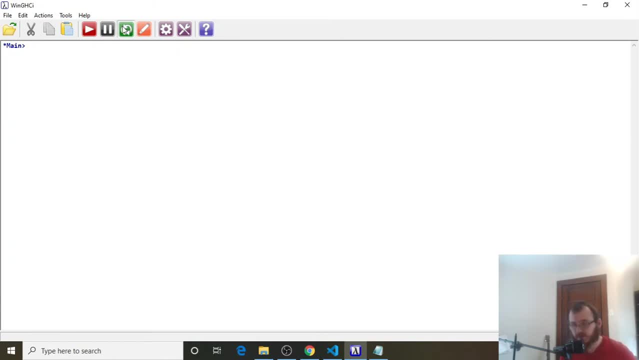 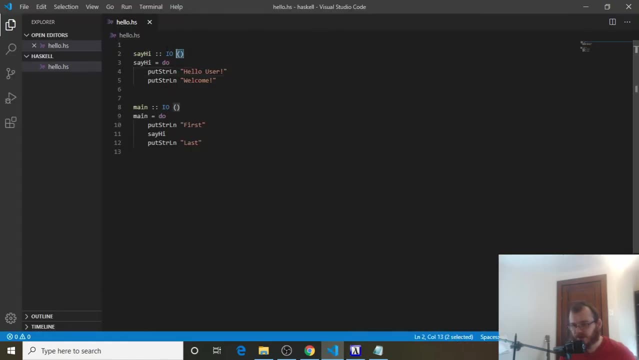 head over to win ghci and we're going to clear it, reload and run and you'll notice we get the exact same results as we did before, but now we've typed out our functions, so we put the types above and it just adds a little bit of clarity to our program so that we can kind of see: 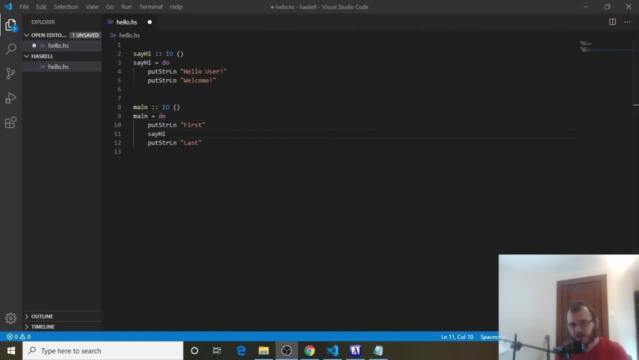 what's going on at first glance and we don't have to guess. now let's talk about calling a function multiple times. so we have the say hi function. we called it once inside a main. what happens if we call it three times? say hi, say hi, say hi. here's the order that it will happen in. 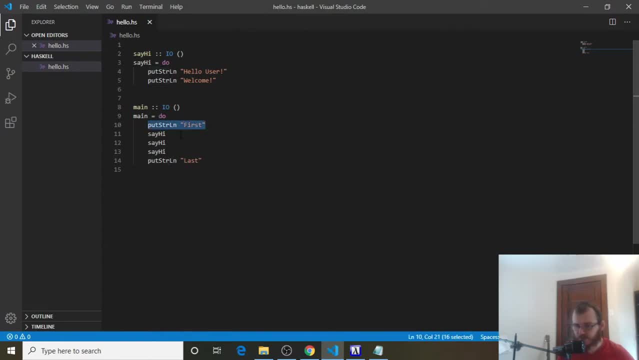 so do runs from top to bottom: main equals. do it puts first, Then it runs the entire say hi function. so it's going to print: put hello user and then welcome. Then it's going to run the second say hi function. It's going to do it again: put hello user and welcome, and then it's going to run it again and for a third time put 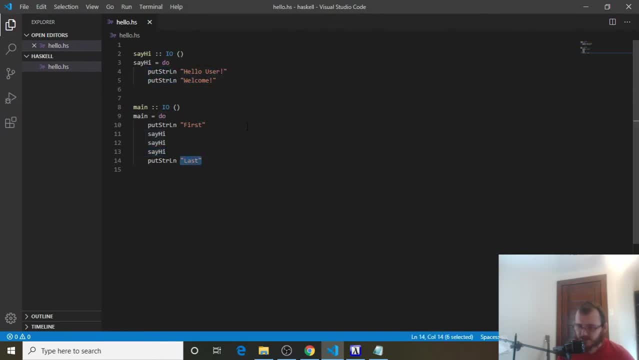 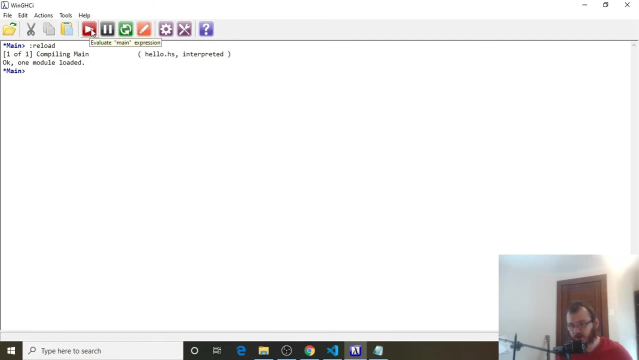 Hello, user and welcome. and then, finally, it's going to put this last to the console, right? so let's save it, go over to win ghci, clear it, reload and Evaluate it and you're going to see: this is the first say hi, This is the second say hi and this is the third say hi, call for the function, right so? 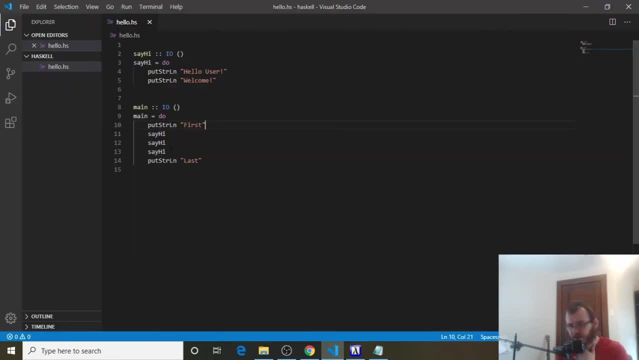 This can come in, really come in handy in that we can take this logic out instead of doing this three times. This is a little harder to read, right? so instead of doing that, we took that logic, put it inside of say hi, and Then we just called say hi inside of mean, and it looks a lot cleaner. 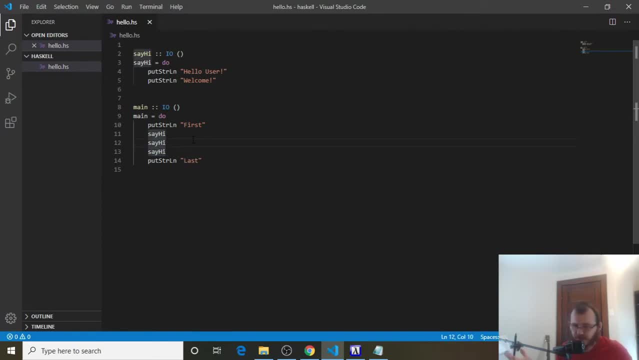 And it's just a lot nicer To read and, yeah, it's a lot easier to read, so let's keep going. So now we're going to talk about passing a parameter to our function, so we're going to get rid of the to say hi's and just leave one, and 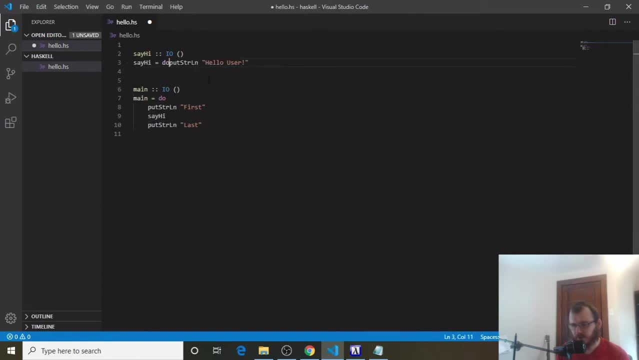 Then up top here We're just going to leave: put string Ln- Hello user. so this will run first it'll put hello user and then it'll run last. But now we want to pass a parameter. Let's say, instead of hello user, We want to greet the user by their name. 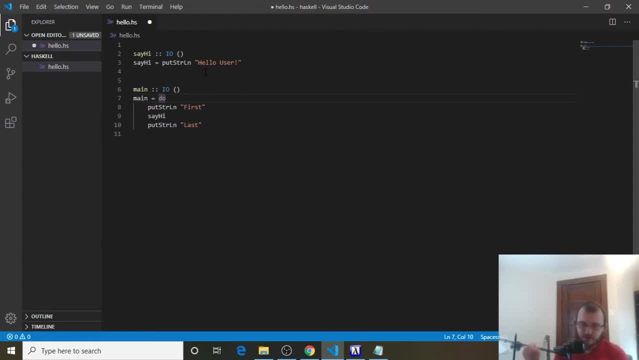 So we can pass what's called a parameter into our function and do our say hi function And then we can say hello and use that like as a variable and say hello name. so to do that For say hi, we're gonna go on the left hand side here and if we want to pass something in to say hi, 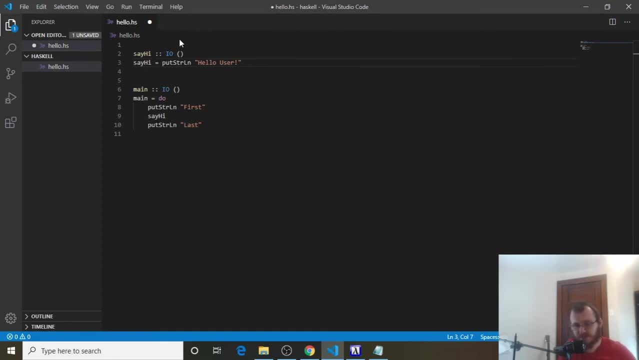 On the left hand side. We're going to leave a space and then we're going to pass the parameters. So in this case, we want to call it name, We want to pass a name in to say hi, so So say hi, and it's going to take in somebody's name: George, Mike, Tom, Jill, Anna, Anna, anything like that. 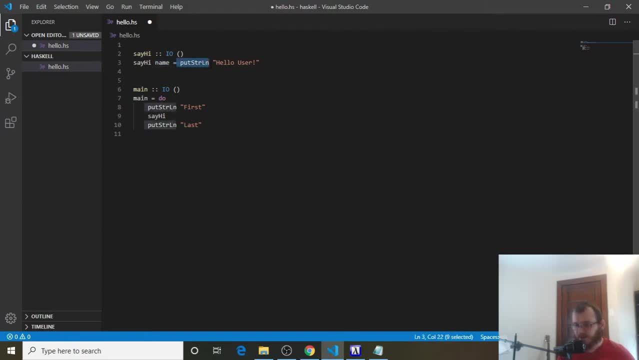 And on the right-hand side it's going to put to the console and remember our string concatenation. so we could do something like: instead of hello user, we could have a string of hello space plus plus name, And in this case, remember variables. instead of saying in do, instead of saying let name equal something. 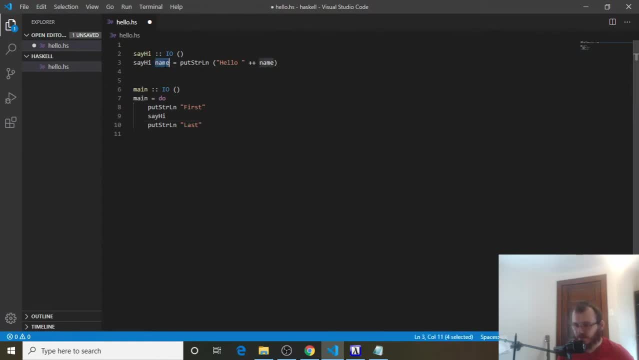 we're saying, hey, here's the name that we're passing in and we're going to print out hello and the name we passed in, And now that we have that, we need to slightly change what is our function signature. So we're still putting something right. We're still putting something to the console. so that's that IO part. 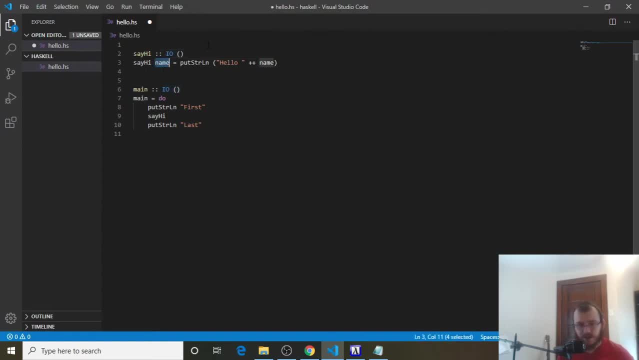 Now, before that, we're passing in a name, right, And a name is going to be some type of string, And to do that, and we need to change our function signature, so we need two parts to our function signature. now We need to tell it that, hey, the last thing we're going to do is put something to the console. remember, that's the IO part. 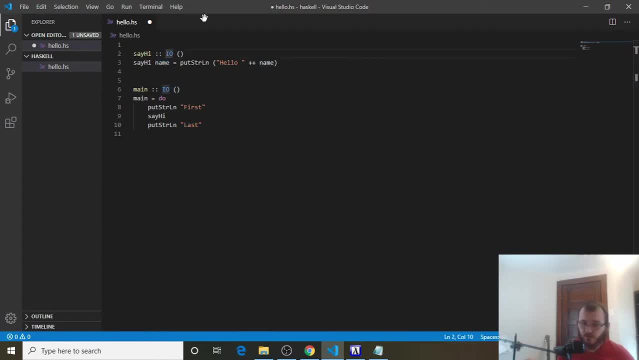 but we're also passing in a name and we're going to put that before we. we're going to pass in a name and then we're going to put something to the console and the name we know is going to be a string. 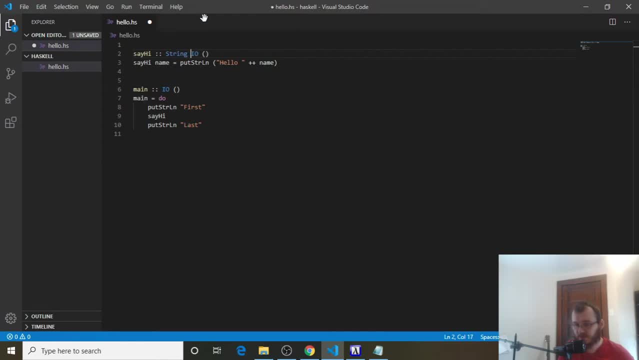 So type string like this: and then we're going to add an arrow- Remember the arrows from before, but they went the other way- and we're going to add an arrow and we're going to say, hey, we're going to return or we're going to our. last part of our function is going to put something to the console. 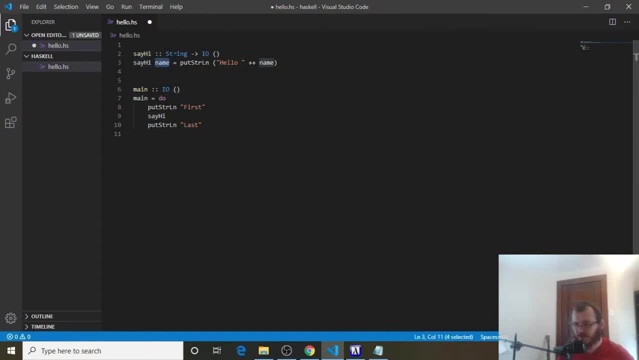 So, one more time, the sayHi function takes in this name parameter. it's going to be a string and it's going to return, or it's going to. the last thing it's going to do is put something to the console, which is this bit: 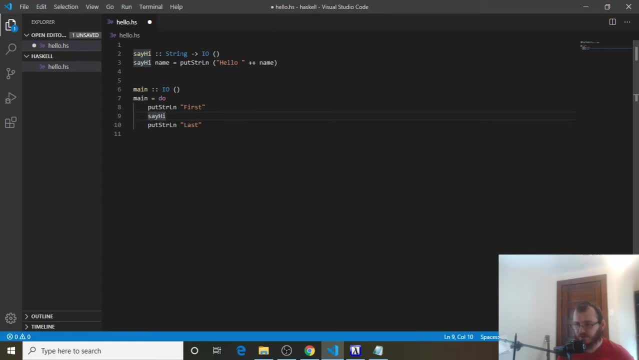 Now down here we can't just do sayHi anymore. If we try and run that it's expecting you to sayHi to someone and to do that, we put a space, just like we did putStringLn right. 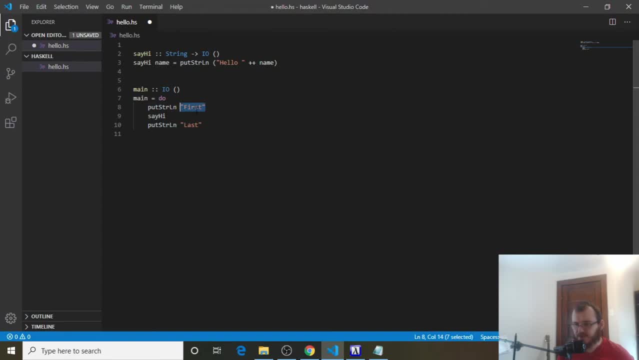 We've used parameters before We've actually passed. first, this is the parameter for putStringLn. last is the parameter for putStringLn, and we pass parameters into print. We've seen these before, but now we're using our own custom function, right? 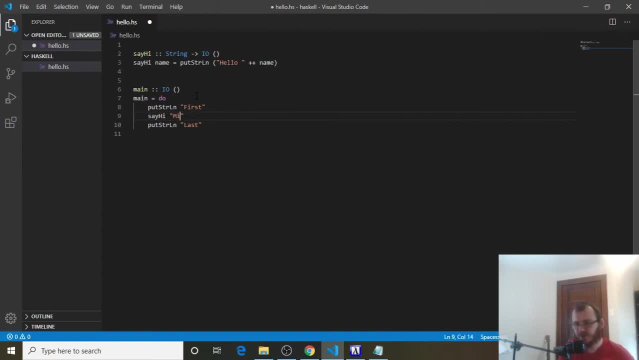 So we still put the space and we want to put someone's name, so Mike. And now we're going to sayHi to Mike, so let's save it control-s. so Mike goes in, name becomes Mike, and then we put hello++ and we know name is Mike, so it's going to be helloMike. 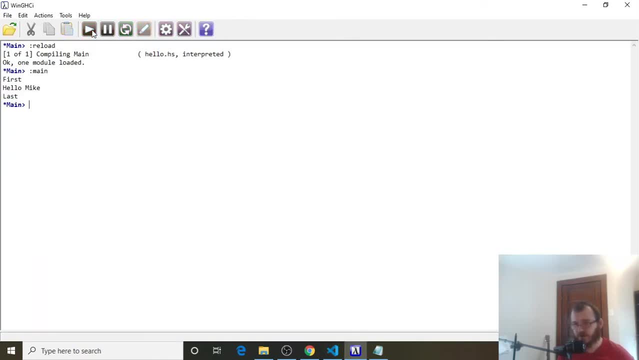 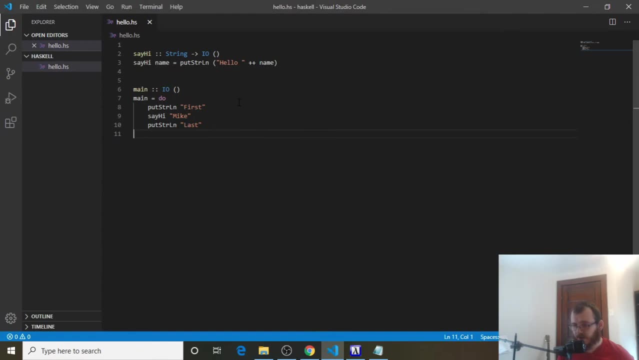 Let's go over here, clear it, reload and run it and it's going to say: first, helloMike, last. Okay, back we go. Now let's suppose we want to sayHi to multiple people. right, We can do that. This is the beauty of parameters. 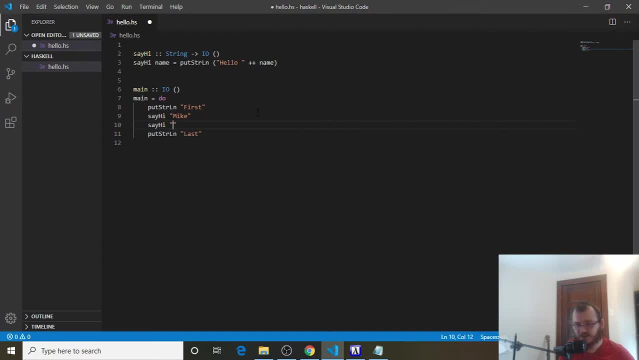 So we can do sayHi space, and instead of Mike, let's do Anna, and let's sayHi to a third person, Elsa. So there we go. Now we're going to sayHi to Mike, Anna and Elsa. 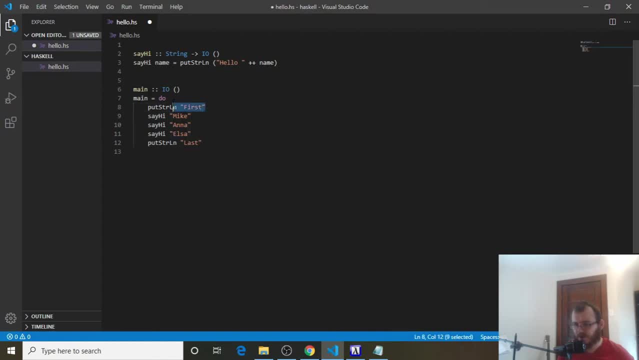 So the first time, here's what happens, right: We run main first gets put to the console. then we run sayHi with Mike as the parameter. so Mike goes in as name and then we put to the console: helloMike. 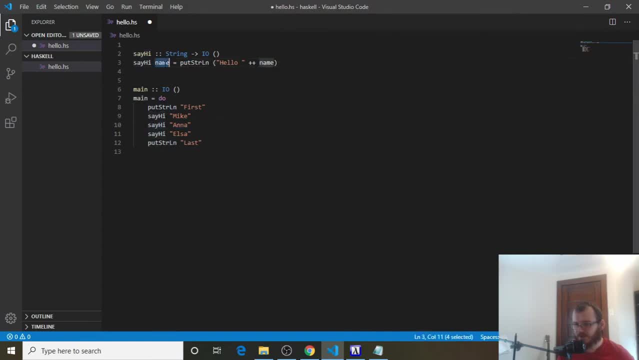 Now we run sayHi again with Anna. Anna comes in as the name we put to the console, helloAnna. Elsa comes in to sayHi, and then we do putStringLn helloElsa, And then, finally, we put the name into the console: helloElsa. 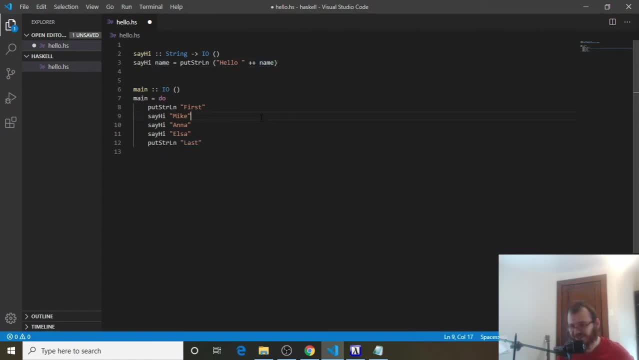 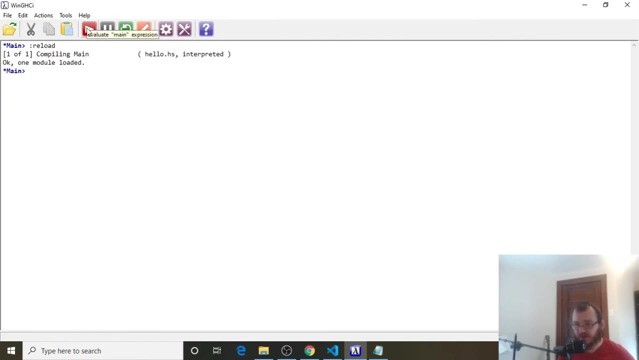 And then finally we put the name into the console: helloElsa. And then finally we put loss. And then finally we put loss, So loss, So control-Less to save, And we go over to WinGHCi: clear it, reload and evaluate. 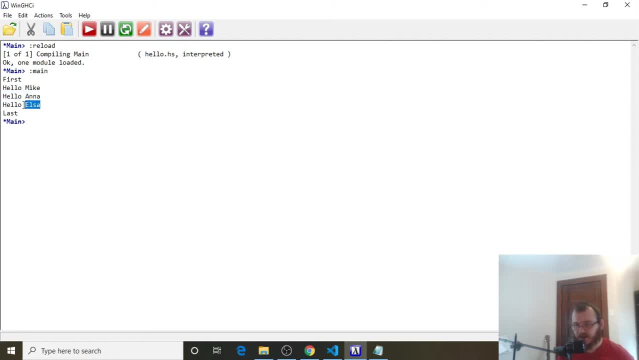 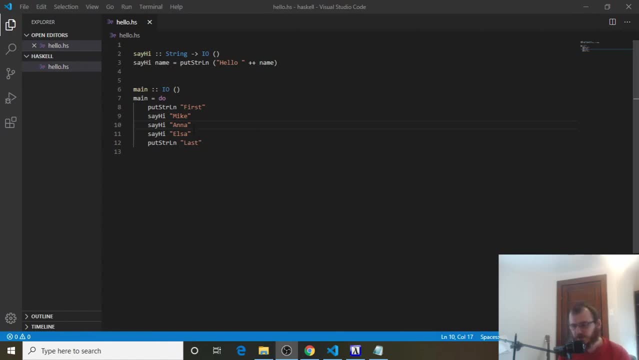 And you're going to see: first, helloMike, helloAnna, helloElsa loss. So now let's talk about passing multiple parameters to a function. So we're going to leave this be for now. We're going to come up here to this: sayHi. and now we don't only want to get the name right. 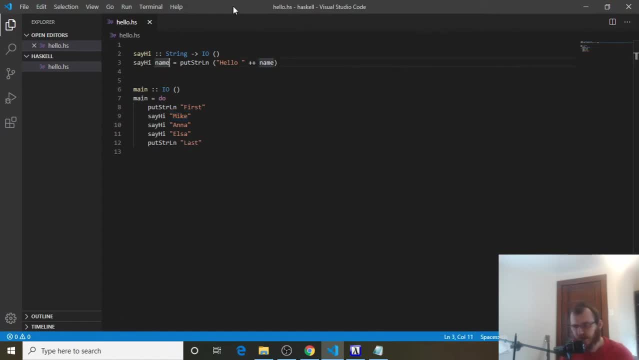 we also want to get an age for each one, an age for each person, so we can say name space age. so now we have this: say hi, name for the function and we pass in a name and an age on the left hand side. those are our parameters: name and. 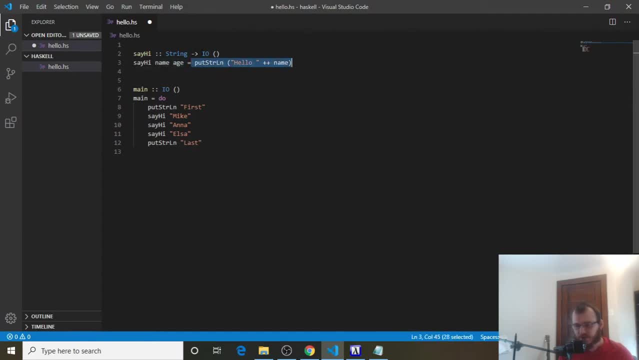 age. then, on the right hand side, we still put something to the console, in this case a string. right, we put a string to the console, and so now we need to change our function signature to match these parameters, and what that means is: name was a string, and now we're also passing in an age and 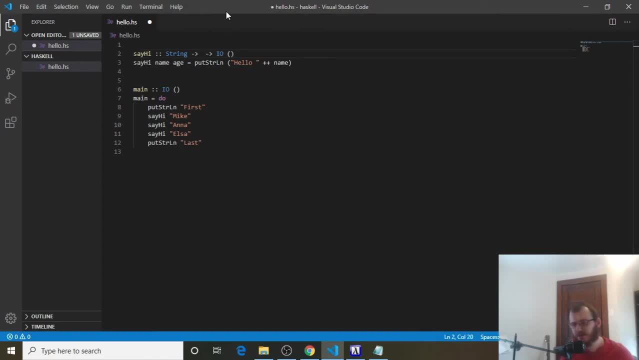 an age, in this case is going to be an int right, some type of number. so age is int. and then, once we've covered our parameter- so name is string, age is int. notice: we go in order and then we tell the function signature what the result is. on the right hand side, in this case, we're putting something to. 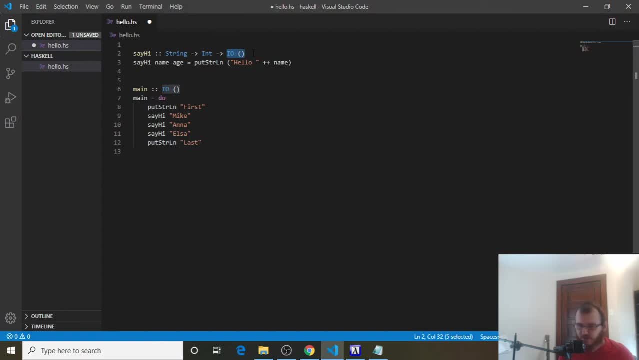 the console and we know that the the the right type for that is io and the parentheses there right. so this is our new function with two new, with a new parameter of age, and we need to be able to use the age on the right hand side, right. 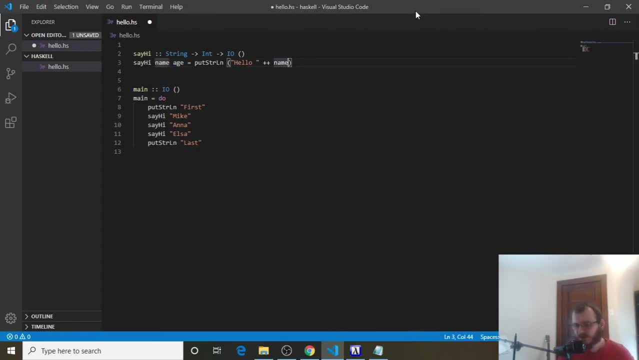 we don't want to just pass age in and not use it so we can say put string all in, hello plus plus name. so hello, in this case it would be mike first and then plus plus, and then we're going to add a plus plus age. now we can't just use age because inside of put string ln- we know put can't do a. 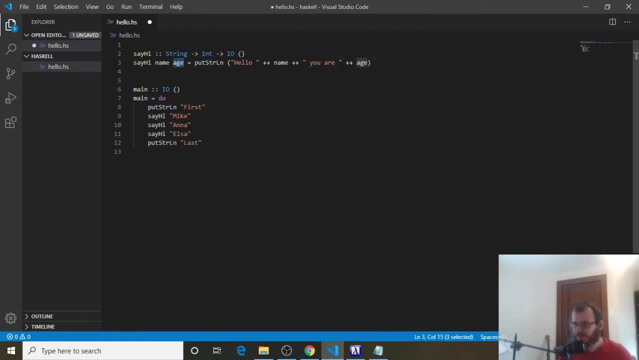 number and in this case a number is coming in. the age is a number and we had a built-in function we used before called show, so we can do show age and that'll say, hey, take this number and we want to turn it into a string so we can put it to the console. so inside of this concatenation we're 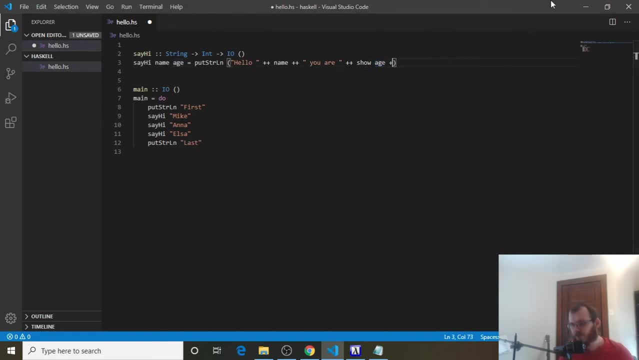 passing age to show, just like we've done before, plus plus years old. so one more time we pass in name and age into say hi, and then we put string, we concatenate everything together. hello name in this case will be mike. you are and then we whatever the age that. 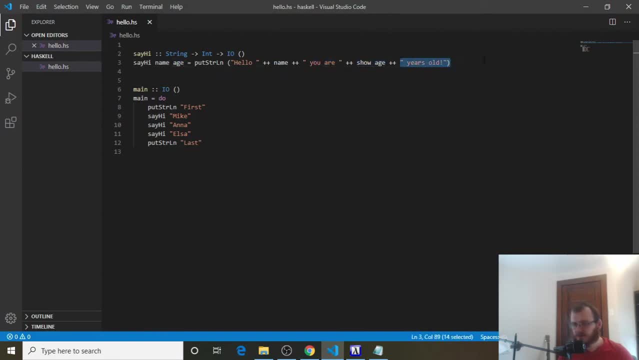 was passed in. we want to show that age is a string and then years old and our new function- signature, right name string age is an int and the last thing we do in say hi is we put something to the console and that's this io parentheses. so down here now, if we try and run this, we're missing an age. we're missing an age for say hi.